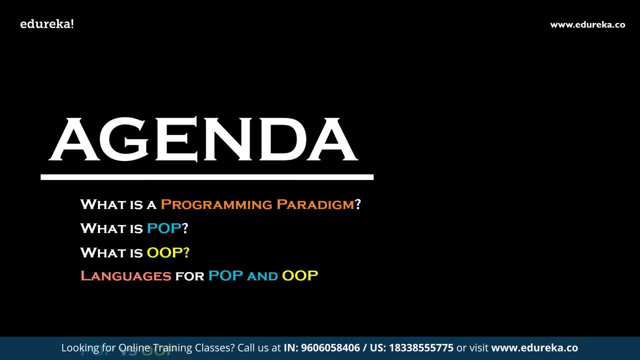 To begin with, we shall first understand what exactly is a programming paradigm, and then we shall throw some light on procedure-oriented programming and object-oriented programming. Finally, we'll be taking a look at the differences between them, based on various factors. So before we begin, 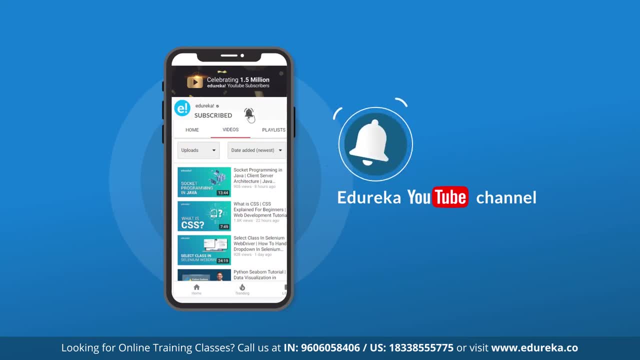 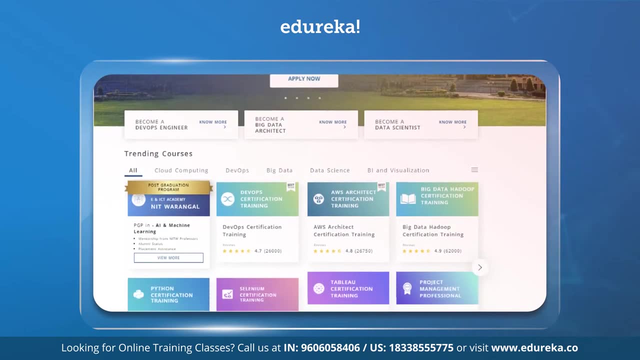 just make sure you subscribe to our channel and hit the bell icon to stay updated with all the latest Edureka videos. Also, if you are interested in getting an online training certification in any of the training technologies, check out the link given in the description box below. 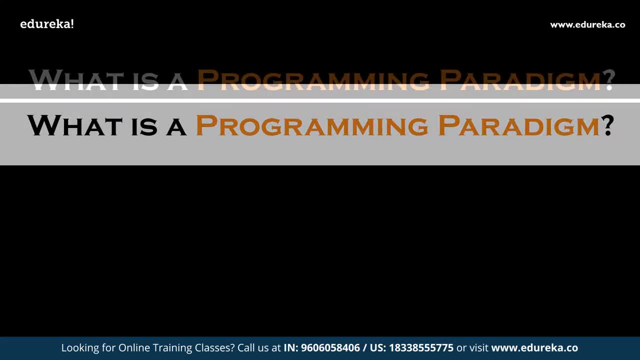 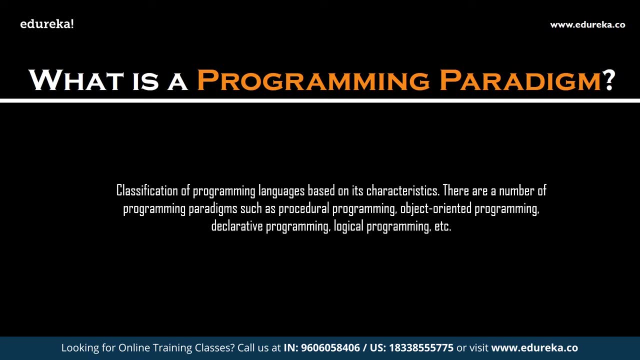 So, coming back towards the session, what exactly is a programming paradigm? Programming paradigm is nothing but classification of programming languages based on their characteristics. There are a number of programming paradigms, such as procedural programming, object-oriented programming, declarative programming, logical programming. 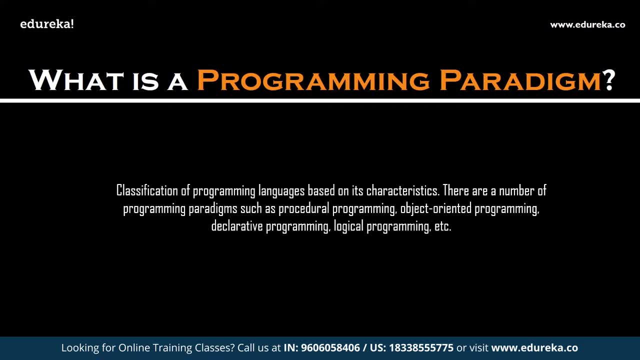 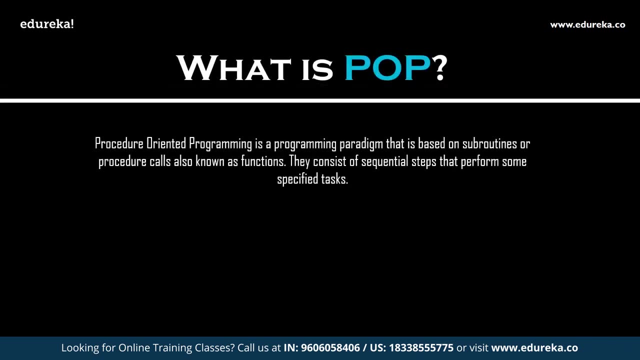 programming, etc. However, the most common programming paradigms are procedural and object-oriented programming. Therefore, every programmer must know what they are and which one suits his project the best. So, talking about procedure-oriented programming, Procedure-oriented programming is a programming paradigm. 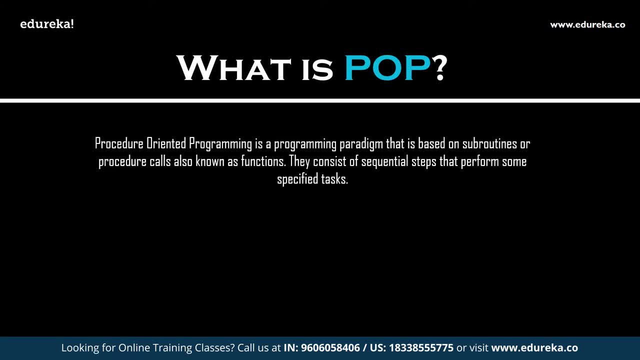 that is based on subroutines or procedure calls. These procedure calls are also known as functions. They consist of sequential steps that are written in order to perform some specified tasks. Therefore, whenever the program requires a function, it requires to perform that particular task. 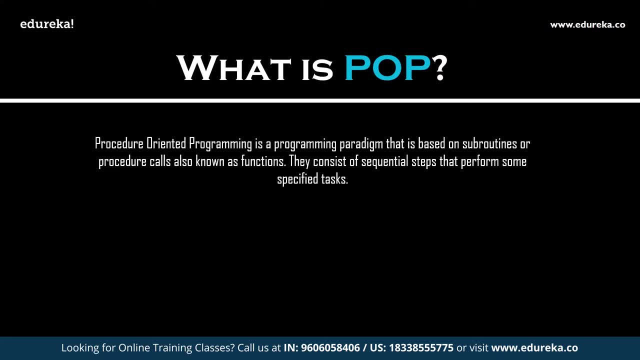 the function will be called. Functions are defined using a unique name. They may or may not have parameters. In case they do, the argument value needs to be passed when the function is invoked or called. To call a function, you will need to make use of the name of the function. 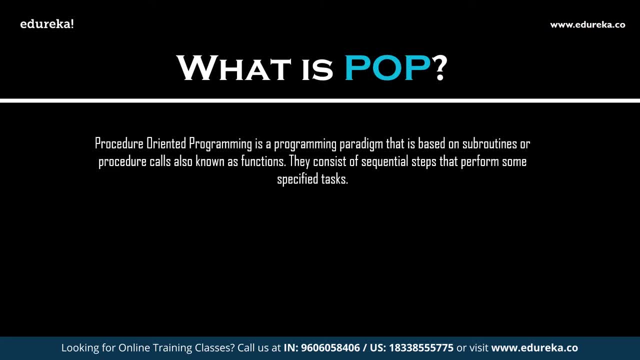 and pass all the necessary parameters. Functions can also return values. In procedure-oriented programming, a function that returns a value needs to have a return type which is of the same type as the type of value that is returned by the function. In case it does not return any value, 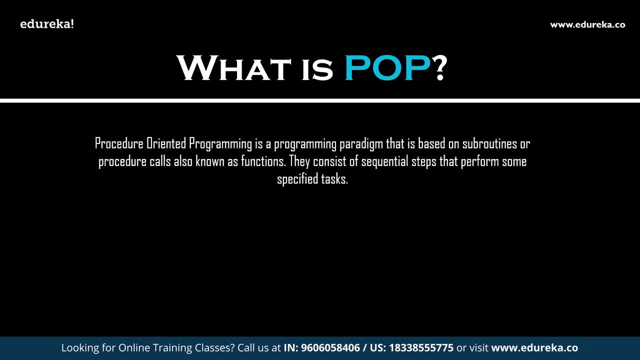 the return type will be void. Procedure-oriented languages were first developed somewhere around the 1950s or 60s. Some of them are ALGOL, COBOL, FORTRAN, BASIC, C, etc. Features of procedural programming: 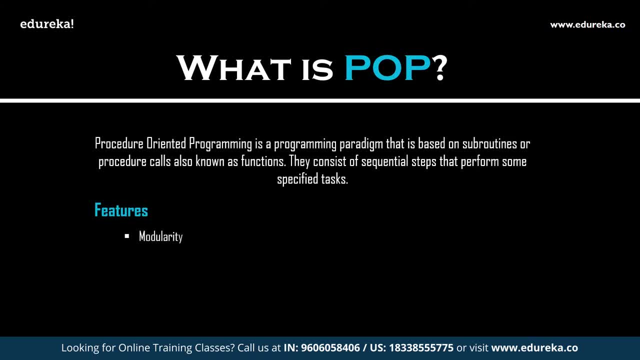 Modularity. Procedure-oriented programming provides modularity that aims to break down complex programs into smaller modules that have single independent tasks. These modules are later combined to perform the major tasks- Predefined functions. Predefined functions are standardized set of instructions defined by a unique name. 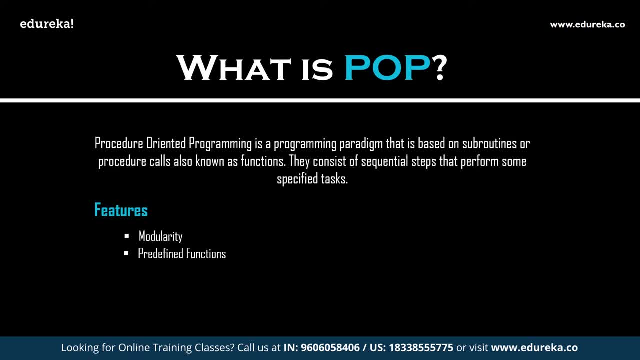 that are designed to perform particular tasks. Some examples of predefined functions in C language are the printf function, scanf function, gets, puts, etc. Scoping: Scoping refers to the area within a program where named entities, such as a variable, can be accessed or used. 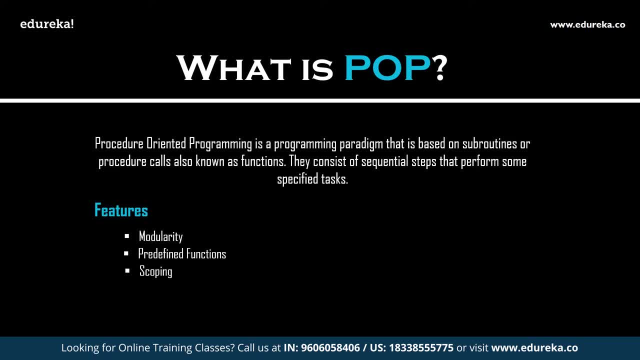 Scoping can be either local or global. Local variables are basically defined within a function or a loop. These variables can be used only within that region, that is, within the function or the loop wherever they are defined. Using them anywhere besides this would result in an error. 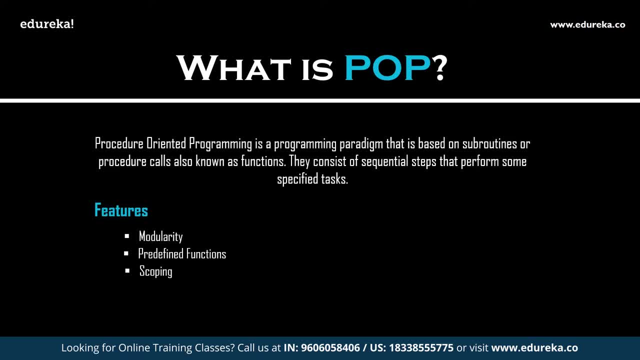 Therefore, variables specific to a function can be prevented from being used by another function. Different functions can have their local variables with the same name. Say, for example, in a calculator program function called add has a variable named a Another function, such as subtract. 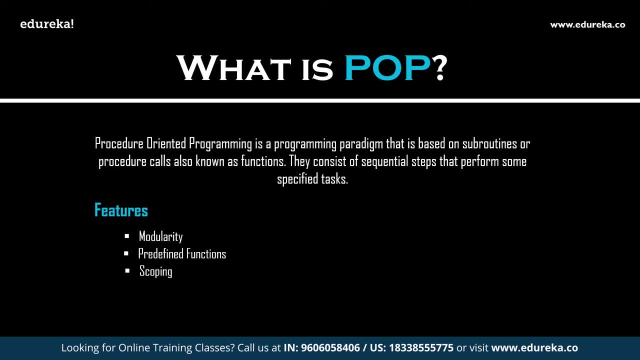 can also have a variable named a. Local variables are created when the function is invoked or called, and they are destroyed when the function has been executed. Therefore, there will be no need to manually delete unnecessary variables. Also, the values of local variables cannot be modified by other functions. 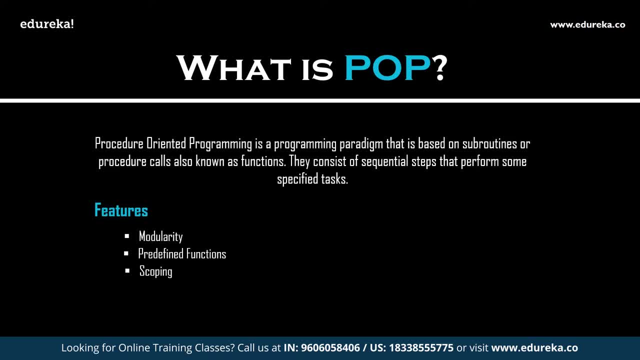 Global variables, on the other hand, are defined within the program body, outside the procedures or functions. Unlike local variables, global variables can be used anywhere throughout the program. Using global variables helps you refrain from supplying same values over and over again, thereby increasing reusability. 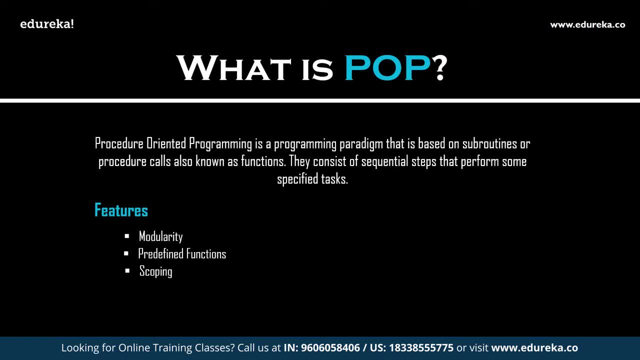 Any function present in the program can access global variables, but when you use them you must be careful, because their values can be modified by functions. Parameter passing. Parameter passing is a technique that is used to pass parameters or arguments to a function. It can be of any type, such as pass by value. 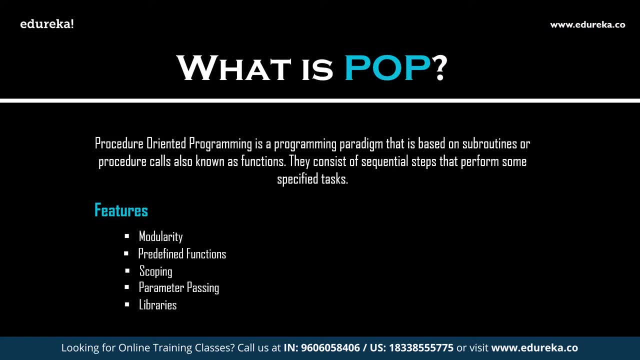 pass by reference, etc. Libraries. Libraries are nothing but collections of predefined functions, classes, codes etc that can be used to pass parameters. This is a technique that can be used to pass parameters etc. within any program. Some of the libraries that are present in C language. 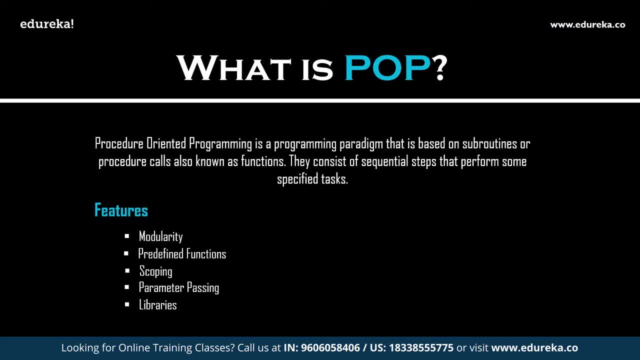 are standard input-output library, the string library, etc. Okay, so now talking about the advantages of procedural programming. In procedural programming, source code is portable. This means codes that is written once can be used on different systems. You can write any type of programs. 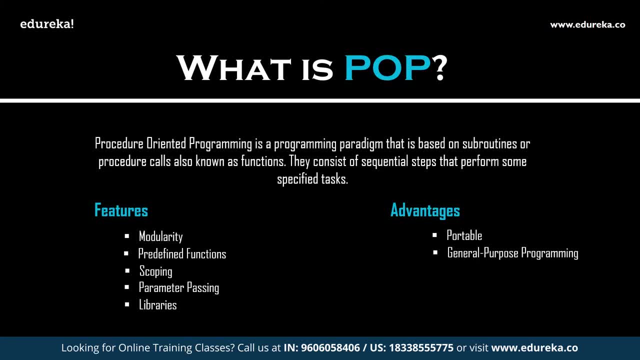 using procedural languages. Therefore, it is very good for general purpose programming. Procedural programming also reduces code redundancy through functions. A function that is once written can be used anywhere throughout the program. A reduced code also leads to reduction in memory usage. 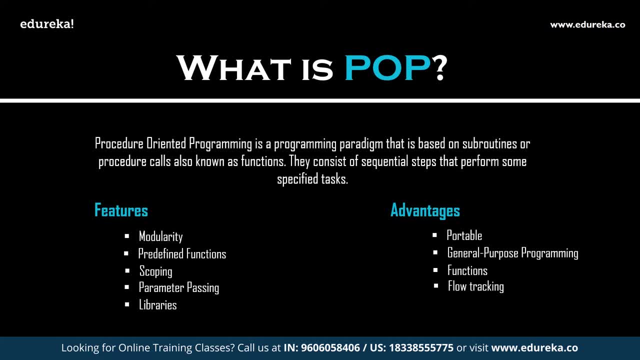 You can easily track the flow of the program at any point in execution. Also, a large number of study materials are available online and offline that can help you learn procedural programming easily. Now, there are a few disadvantages of procedural programming as well When it comes to large-scale project development. 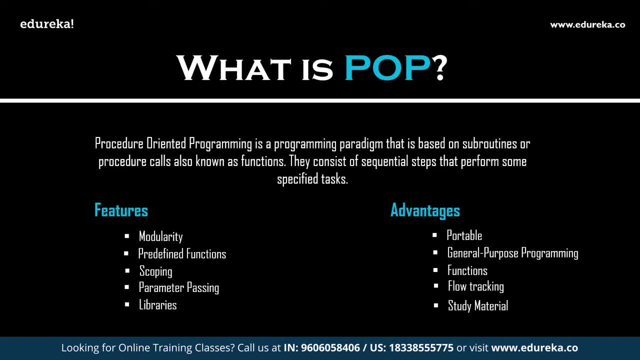 the code is not very much reusable. Therefore it increases the time and effort required to build large-scale applications. It is also not possible to write code by relating to real-world entities. Procedural programming is not recommended for data-sensitive projects, as it does not really focus on securing the data. 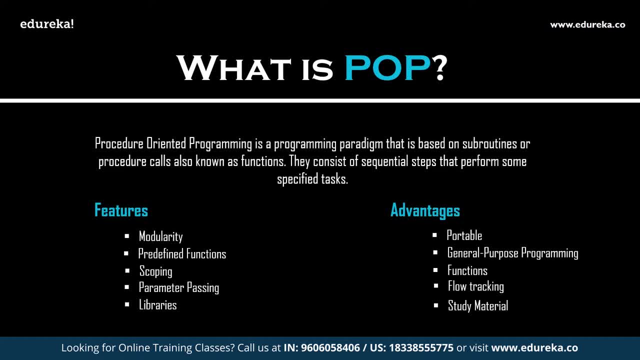 As the size of the code increases, it becomes more and more difficult to manage the code. Automatic memory management is also not available. So by now I hope you've understood what is procedural programming and the basic advantages of procedural programming. Now let's move on. 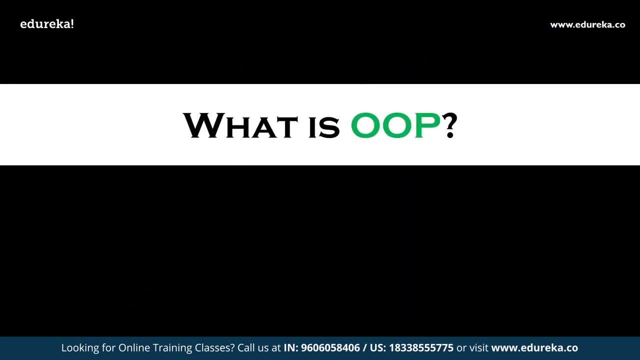 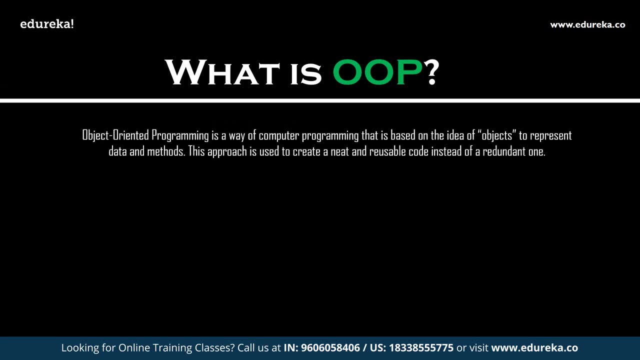 and understand what is object-oriented programming. So, talking about object-oriented programming, Object-oriented programming is a way of computer programming that is based on the idea of objects to represent the data and methods. This approach is used to create a neat and reusable code instead of a redundant one. 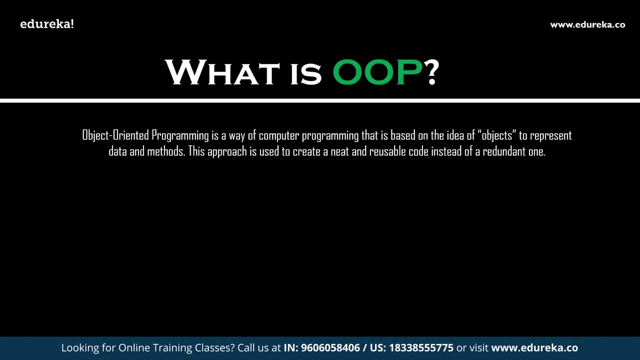 The program is divided into self-contained objects or several mini programs. Every individual object represents a different part of the application, having its own code. So it is important to understand what is procedural programming and what is object-oriented programming. Now let's move on and understand what is object-oriented programming. 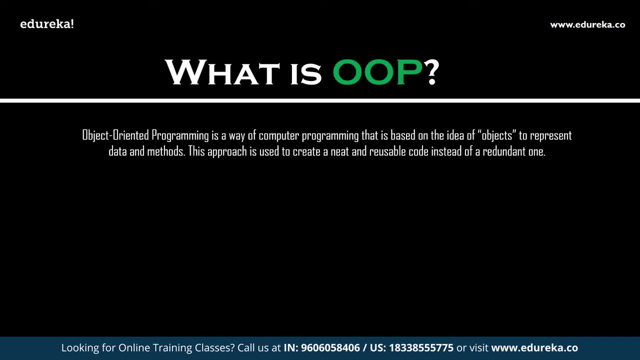 Object-oriented programming is a way of using the same logic and data to communicate within themselves. Okay, so what is an object? An object is a real-world entity such as a pen, book, person, animal, etc. that has a state and some behavior. 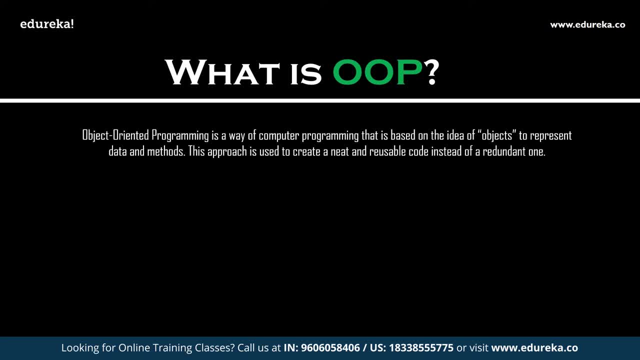 A class is a collection of objects, or you can say that it is a blueprint of objects, defining the common attributes and behaviors. Now the question arises: how do you do that? Well, it logically groups the data in such a way that the code reusability becomes easy. 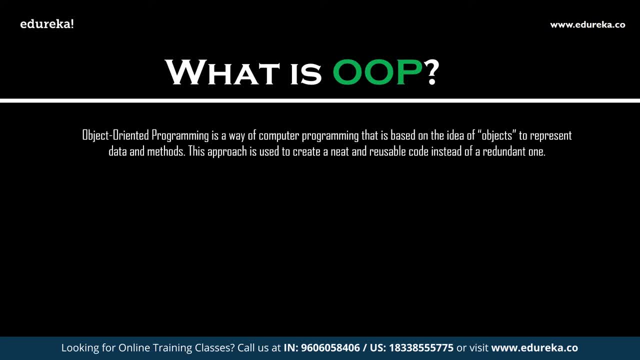 I can give you a real-life example. Think of an office-going employee as a class and all the attributes related to him, like employee name, employee age, salary ID, etc. as its objects. So the employee class basically combines all the data. 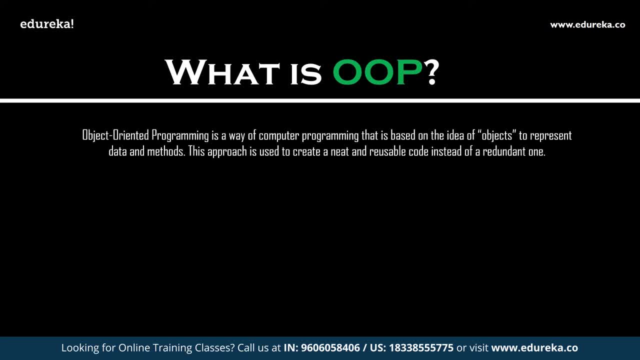 and the code that is needed to work on that data. Classes are defined using the class keyword. So what exactly is the difference between a class and an object? An object is a real-world entity which is an instance of a class. A class is basically a template. 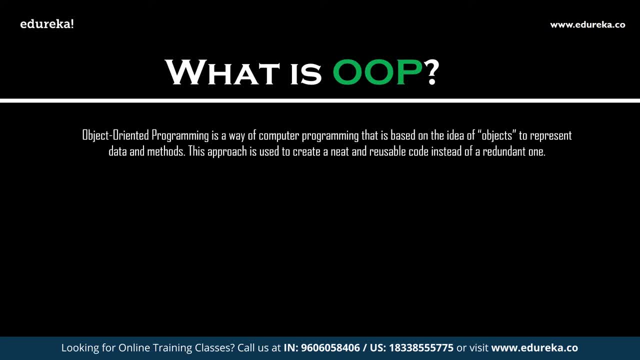 or the blueprint within which objects can be created. An object acts like a variable of a class. Class, on the other hand, binds methods and data together into a single unit. An object is a physical entity, whereas a class is a logical entity. 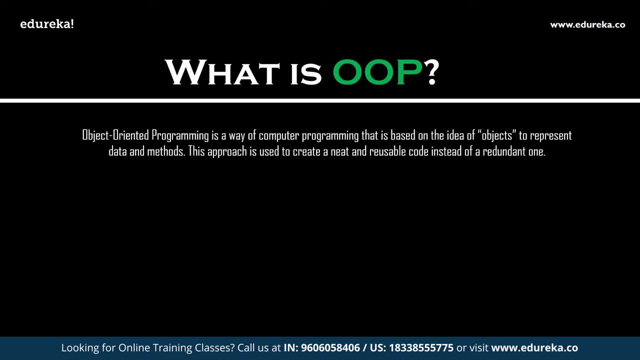 Objects take memory space when they are created. A class does not take any memory space when it is created. Objects can be declared as and when required and, on the other hand, classes are declared just once. Advantages of OOPS: Object-oriented programming allows clarity in programming. 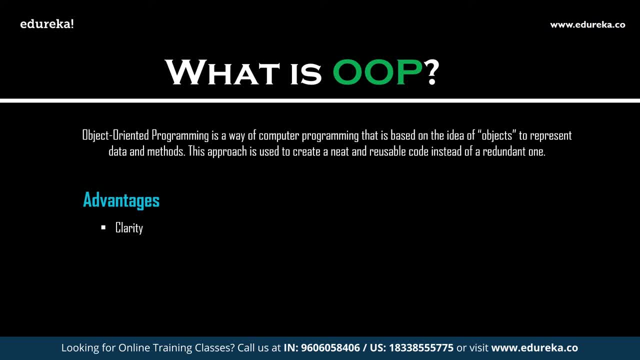 thereby allowing simplicity in solving complex problems. Code can be reused through inheritance, thereby reducing redundancy. The data and the code are bound together by encapsulation. Object-oriented programming allows data hiding, Therefore private data is kept confidential. Problems can be divided into different parts. 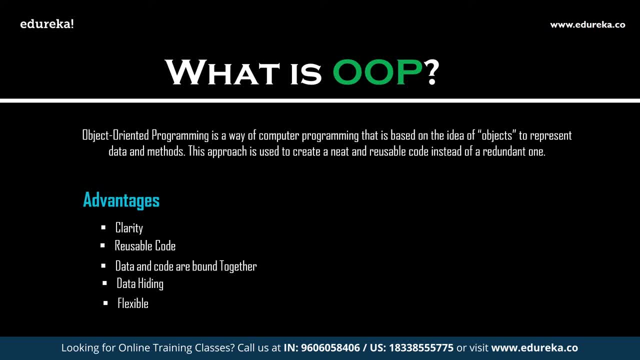 making it simple to solve. The concept of polymorphism gives flexibility to the program by allowing entities to have multiple forms. So what are the features of OOPS? The features or the pillars of OOPS are inheritance, encapsulation, polymorphism and data abstraction. 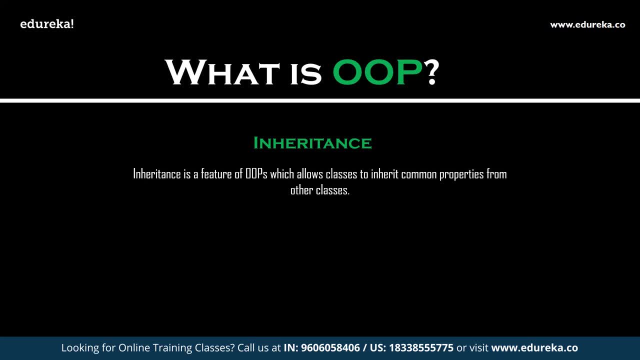 Inheritance is a feature of OOPS which allows classes to inherit common properties from other classes. For example, if there is a class such as a vehicle, other classes like car, bike etc. can inherit common properties from the vehicle class. This property helps you get rid of redundant code. 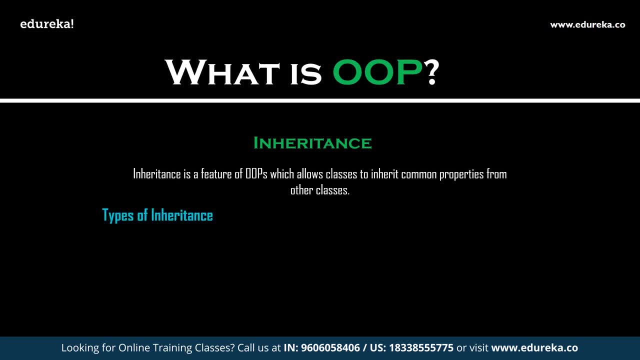 thereby reducing the overall size of the code. There are different types of inheritance, such as single inheritance, multilevel inheritance, hierarchical inheritance and hybrid inheritance. In single inheritance, a single child class inherits from a single parent class. Multiple inheritance occurs when a single child inherits from more than one parent class. 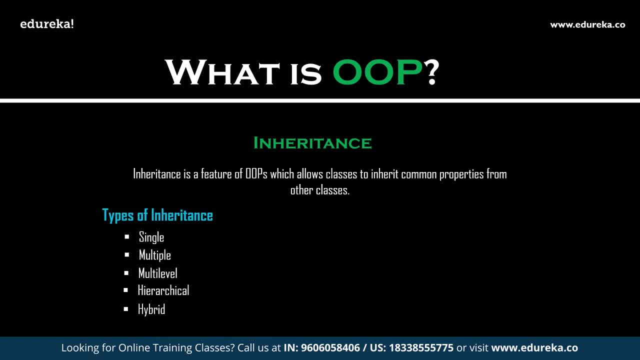 In multilevel inheritance, a parent class is inherited by the child class and that child class is again inherited by another subclass- Hierarchical Inheritance. Hierarchical inheritance refers to the inheritance where one base class has more than one subclasses. For example, the vehicle class can have subclasses. 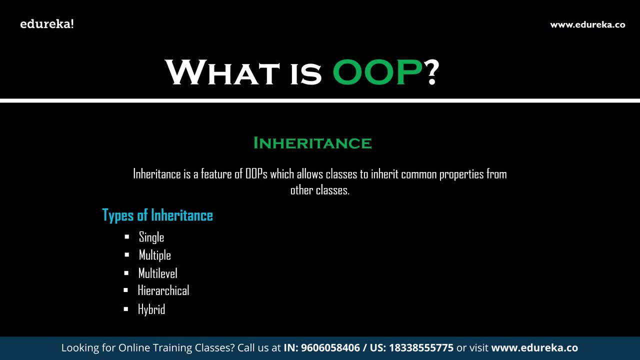 such as car, bike, etc. which again have their own subclasses: Hybrid Inheritance. Hybrid inheritance is a combination of multiple and multilevel inheritance. Inheritance also has some limitations. Inheritance increases the time and effort required to execute a program, as it requires jumping back and forth. 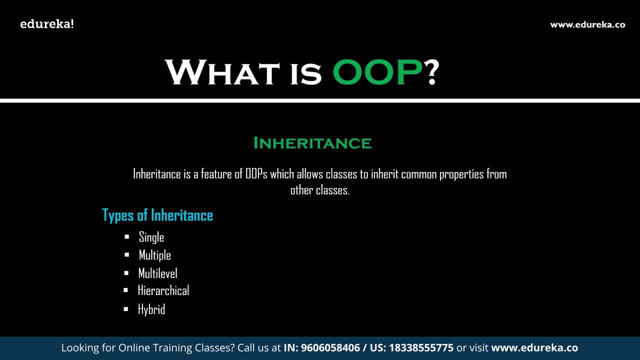 between different classes. The parent class and the child class get tightly coupled. Any modifications to the program would require changes both in the parent as well as the child classes. When you perform inheritance, you'll have to be careful about the implementation, else it would not lead to the correct results. 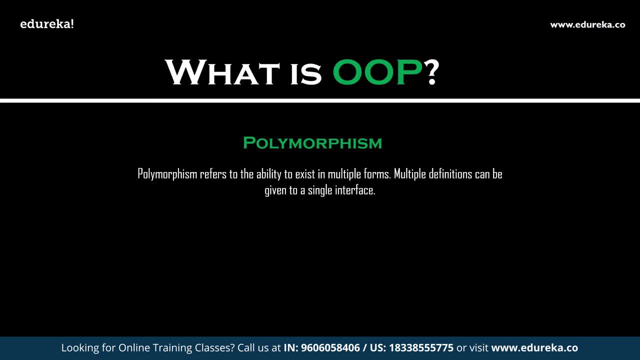 Talking about Polymorphism. Polymorphism refers to the ability to exist in multiple forms. For example, if you have a class named Vehicle, it can have a method named Speed, but you cannot define it because different vehicles have different speed, So all you can do is declare the speed class. 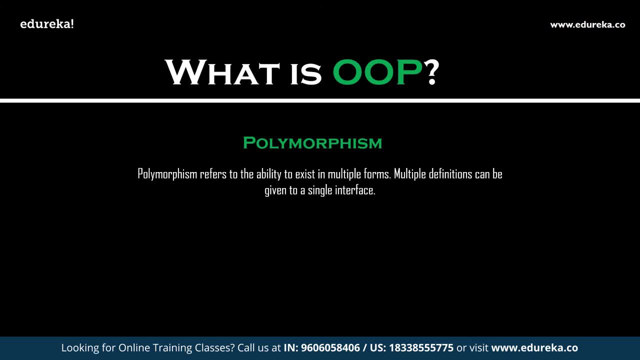 Now the definition of this speed class will be present in the subclasses that inherit the speed class. Types of Polymorphism. Polymorphism can either be static or dynamic. Static Polymorphism, or static binding, is a kind of polymorphism that occurs at compile time. 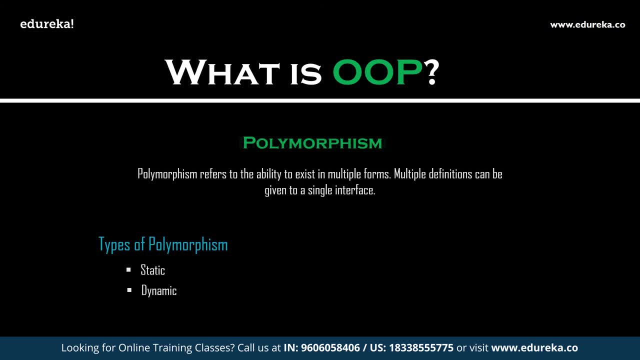 An example of compile time polymorphism is method overloading. Method overloading is a feature of OOPS which makes it possible to give the same name to more than one method within a class if the arguments that are passed differ. Dynamic Polymorphism or Runtime Polymorphism. 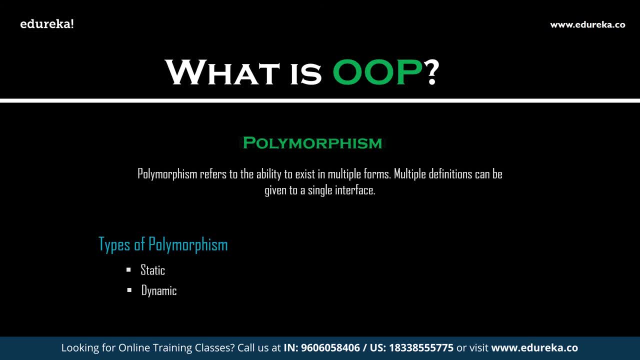 is a type of polymorphism that is resolved during runtime. An example of runtime polymorphism is method overriding. Method overriding is a feature of OOPS, by which the child class or the subclass can redefine methods present in the base class or the parent class. 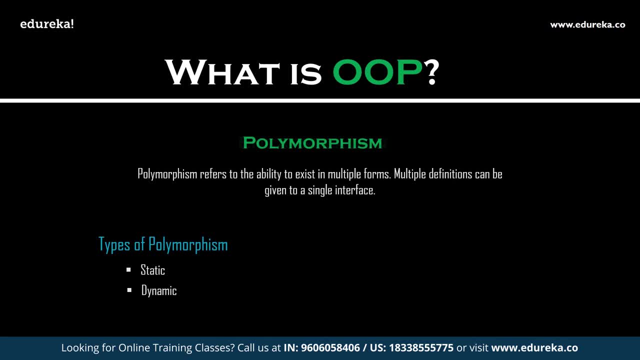 Here the method that is overridden has the same name, as well as the signature, meaning, the arguments passed and the return type. So what is encapsulation? Encapsulation refers to binding the data and the code that works on that together in a single unit. 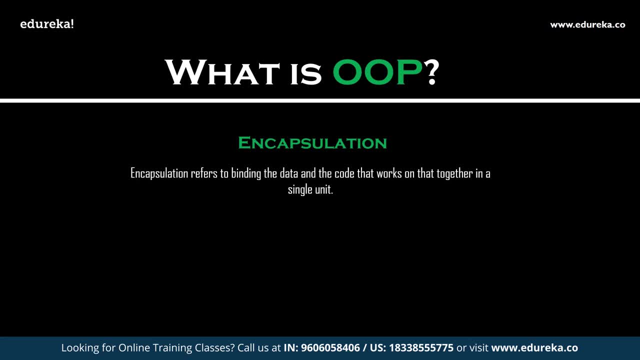 An example of encapsulation is a class. Encapsulation also allows data hiding, as the data specified in one class is hidden from the other classes. This is achieved through access specifiers. Access specifiers or access modifiers are keywords that determine the accessibility of methods. 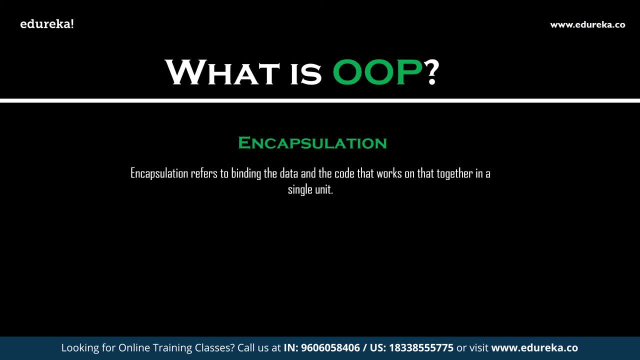 classes, etc. in OOPS, These access specifiers allow the implementation of encapsulation. The most common access specifiers are public, private and protected. However, there are a few more that are specific to the programming languages: Data abstraction. 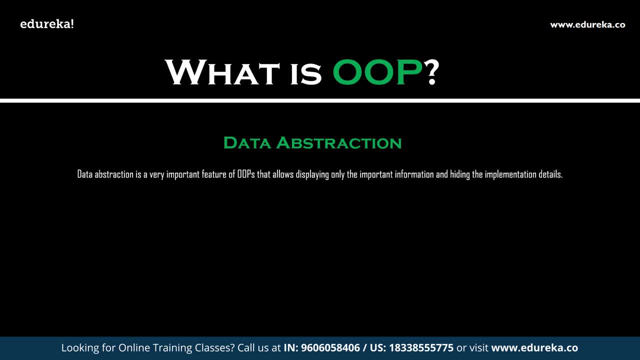 Data abstraction is a very important feature of OOPS. that allows displaying only the important information and hiding the implementation details. For example, when you are riding a bike, you know that if you raise the accelerator, the speed will decrease, But you do not know how it actually happens. 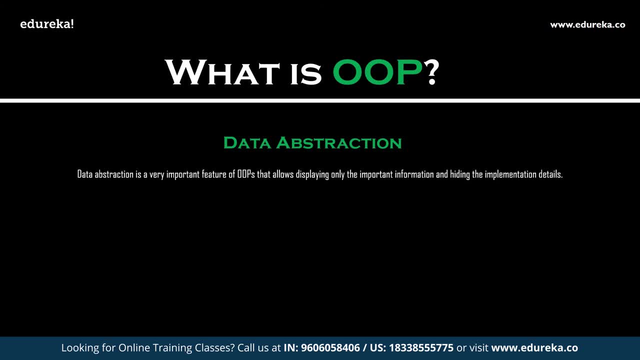 This is data abstraction, as the implementation details are hidden from the rider. Data abstraction can be achieved through abstract classes and abstract methods. An abstract class is a class that contains abstract methods. Abstract methods are basically declared but not defined If these methods are to be used in some subclass. 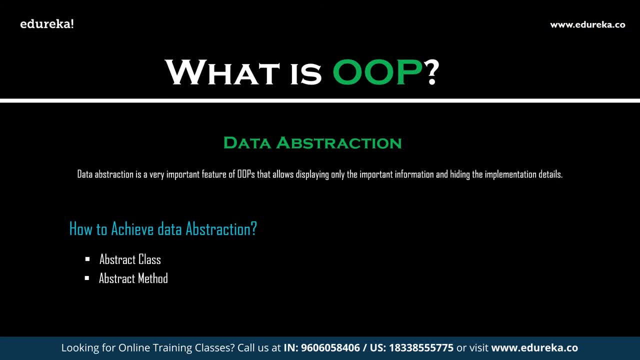 they are to be exclusively defined in that subclass Limitations of OOPS or object-oriented programming. Object-oriented programming is usually not suitable for small problems. It requires intensive testing, takes more time to solve the problem, requires proper planning and it requires that the programmer. 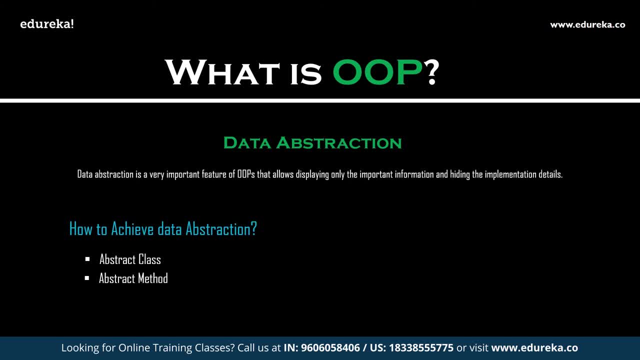 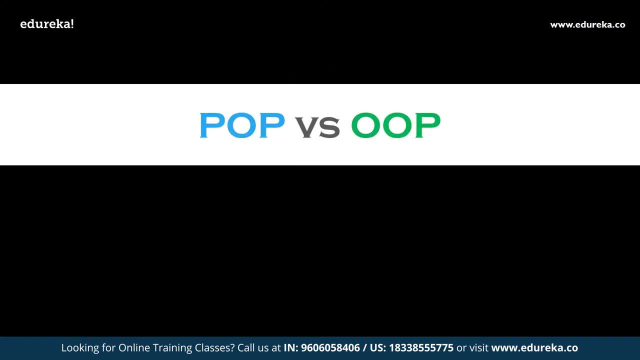 should think of solving the problem in terms of objects. So now that you have a basic idea of procedural programming and object-oriented programming, let's move on and do a head-to-head comparison between them. Problem-solving approach: There are basically two approaches that are used to solve a problem. 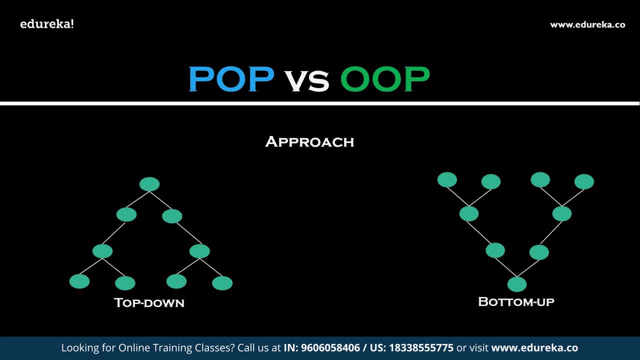 That is the top-down approach and the bottom-up approach. Top-down approach, as the name suggests, begins at the top and moves lower down. So your first deal with the creation of higher level modules and move towards the lower ones. For instance, if you are creating an application to book a flight ticket. 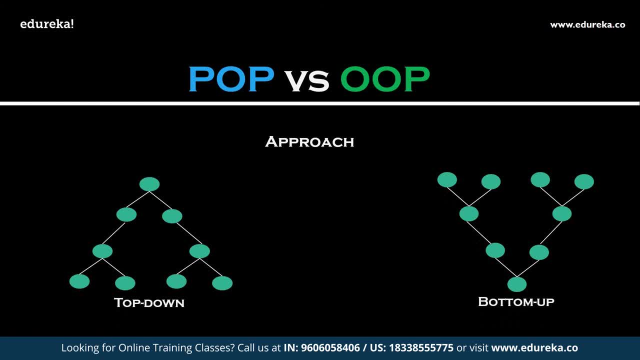 Here, the main concern or the main task is to book a ticket. So you start from here and work your way down towards the subdivisions. Now this problem of booking flight tickets will have sub-parts, like the flights that are available, the destinations, number of tickets. 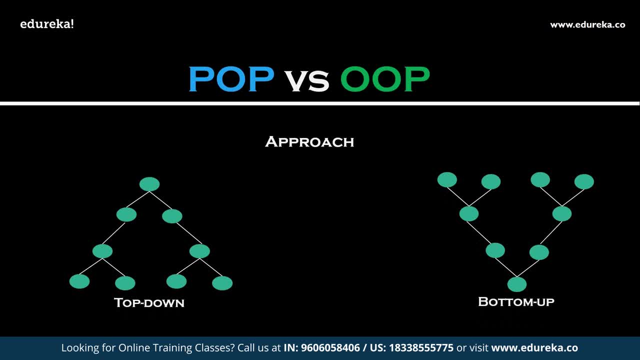 etc. Not just that, even these sub-parts will have further divisions. Bottom-up approach is exactly opposite to this. You begin from the smallest and work your way towards the main problem. The code is much more reusable when it comes to bottom-up approach. 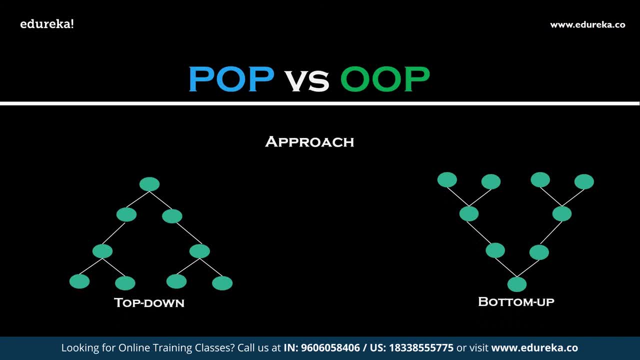 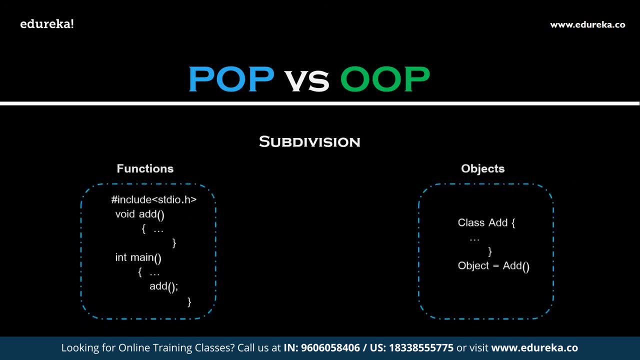 Procedural languages follow the top-down approach, whereas object-oriented languages follow the bottom-up approach. Subdivision: In procedural programming, the program is divided that are created to execute independent tasks. On the other hand, in object-oriented programming, programs are divided into objects. 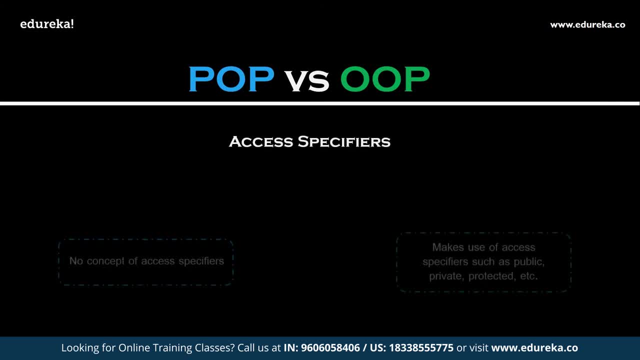 Access specifiers. Access specifiers, as mentioned earlier, determine the accessibility of methods, classes, etc. Procedural programming has no concept of access specifiers, whereas object-oriented languages have access specifiers such as public, private, protected, etc. 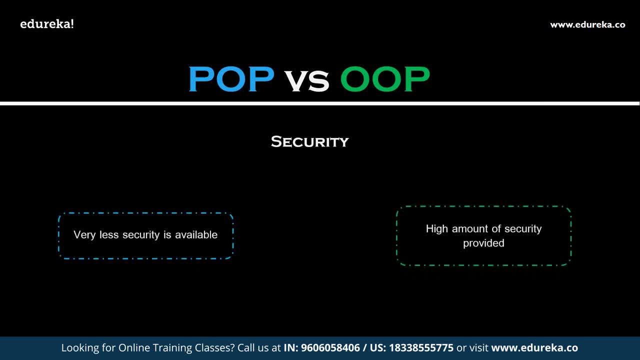 Security. Procedural programming provides some amount of security to the data, as the data present within one function cannot be used by the other function. However, object-oriented programming is very much secure. This is because they make use of access specifiers, as mentioned earlier. 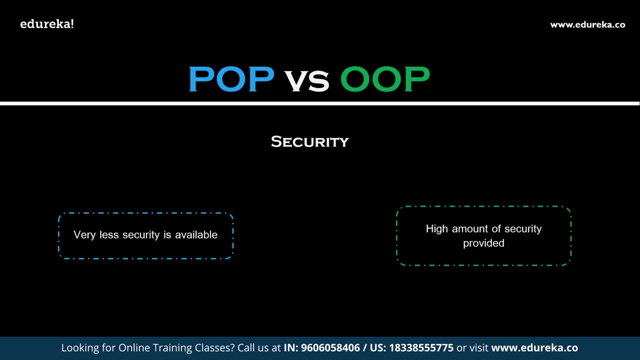 The private access specifier provides maximum security. If you have a class with private members, the data and the functions that are declared private will be private to that class and no other class can access them. Similarly, protected members can be accessed only by the subclasses. 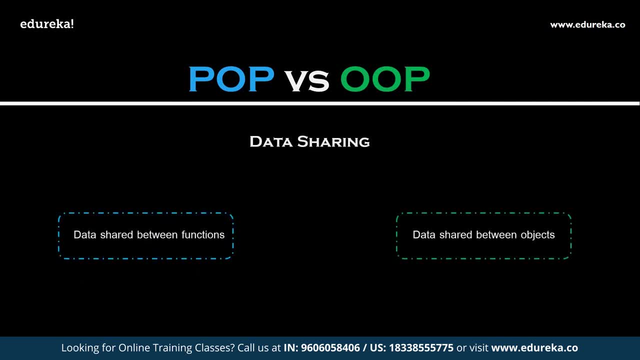 Data sharing. In project-oriented programming, data is shared between functions within a system. On the other hand, in OAPS, the objects can be shared within classes through inheritance Data hiding. Data hiding is a process of combining the data and the functions into a single unit. 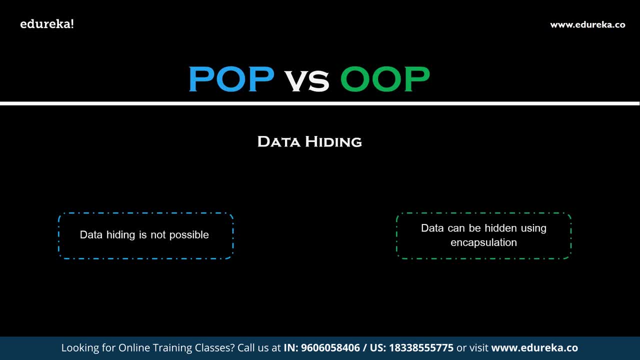 The ideology behind data hiding is to conceal data within a class to prevent its direct access from the outside class. It helps programmers to create classes with unique data sets and functions, avoiding unnecessary penetration from other program classes. In object-oriented programming, data hiding can be easily achieved through encapsulation.